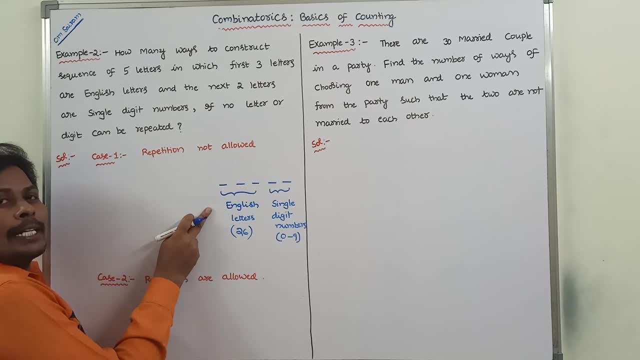 we are using English letters. English letters means English alphabets. So how many number of English alphabet- that is, 26 letters- are there? Okay, next? Next two letters are single digit numbers. So single digit numbers starting from 0 and ending with the 9. So that is 0 to 9. Here. 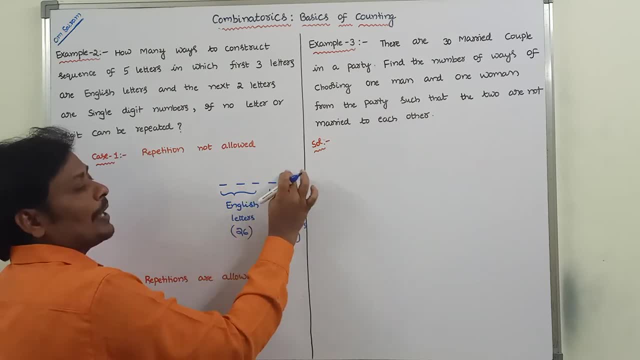 I am using 0 to 9 digits in these two vacant places. Here I am using 26 alphabets in these three vacant places. Okay so, now we go for the problem Solution. Okay so, here in the first vacant place, how many number of letters we have to use? 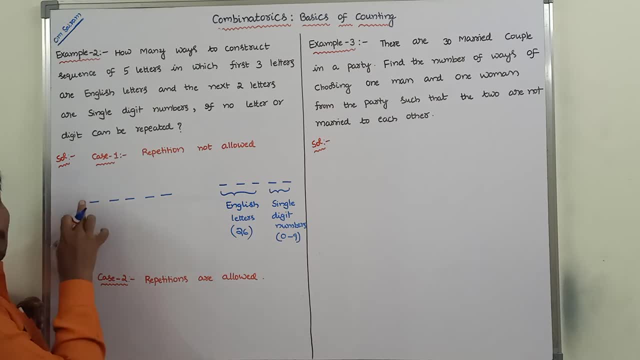 26 letters are used, Either A or B or C or D or E, up to Z. Okay, any letter can be placed in this first vacant place. So there are 26 letters, are there? Okay? how many number of ways? 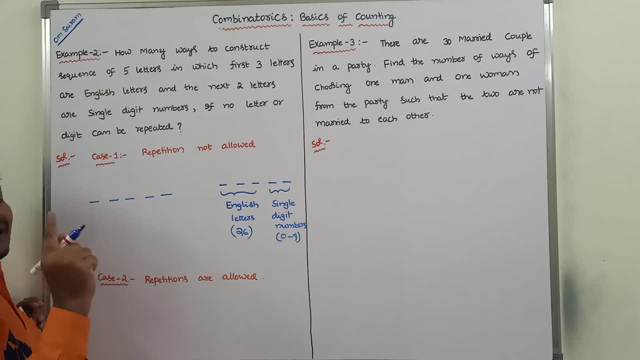 For each and every letter, one way. is there? 26 letters are there? How many number of ways? 26 ways are there? Okay, next one. Next second place. Okay, in the second place. how many number of letters we are using Here? also, 26 letters we are used. Okay, among the 26 letters, one letter. 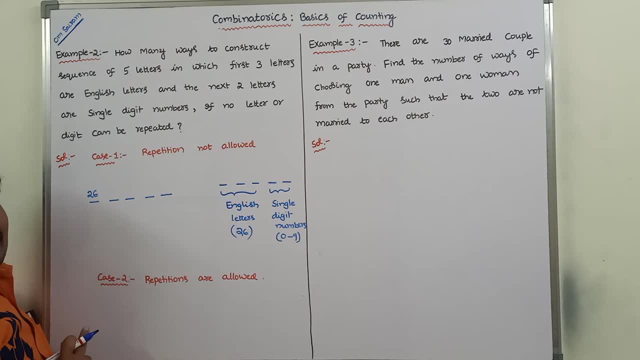 here already filled in. Okay, next one. Okay, in the second place, how many number of letters we are using In first vacant place? Okay, we have to subtract that letter. Okay, so total 26 letters. are there 26 minus 1, that is 25 letters we have to place in this second vacant place because there is no. 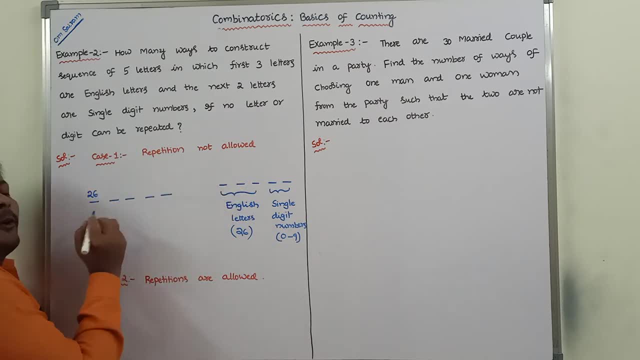 repetition occurred. Okay, so, for each and every letter, one way is there. So 25 into 1, that is 25 ways. Okay, so how many number of letters we have to place in this second vacant place? 26 ways are there to place any letter in this second vacant place? Okay, next. Next third vacant. 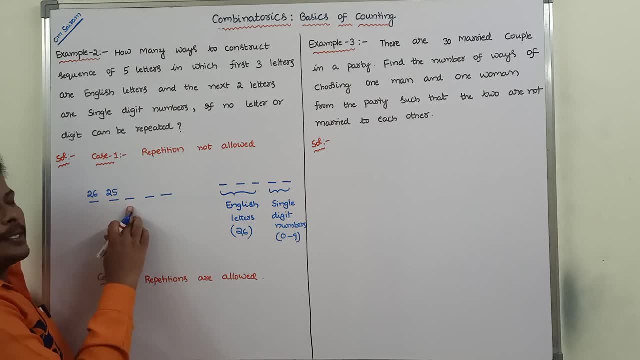 place. Okay, how many number of ways are there So for inserting the English letter? so 26 ways are there. So among the 26 ways, first two vacant places. two letters are already completed, So remaining letters is 24.. 26 minus 2, that is 24 letters are there because there is no repetition. 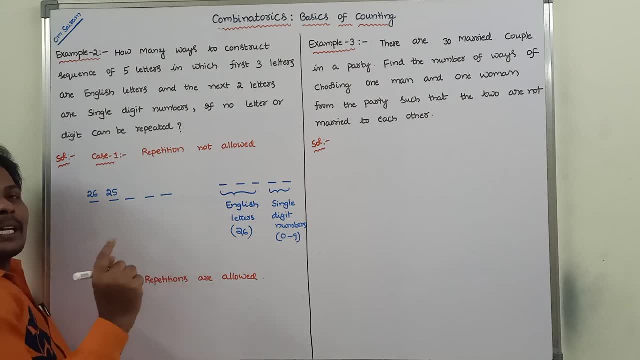 of letters, So 24 letters for each and every letter. here, one vacant place is there. That is one way, is there? So 24 into 1, that is 24 ways, are there? Okay, next one. So here, first three. 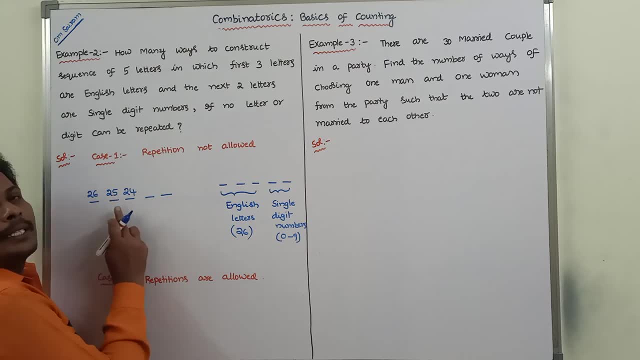 letters are English letters. So it is completed. So here. first, three letters are English letters. So here for filling the first vacant place, 26 letters are there, So for each and every letter. so we have to choose one way. So 26 into 1, that is 26 ways. are there Okay for filling the second? 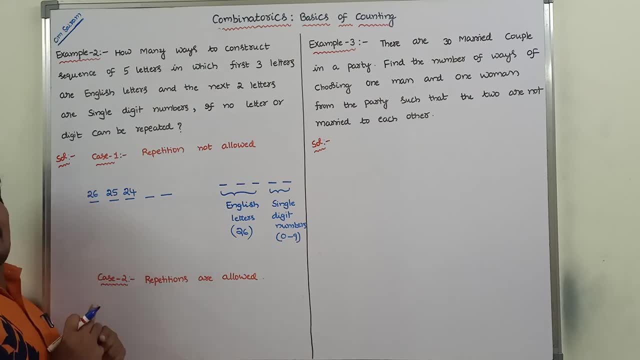 vacant place. okay, only 25 ways are there. because among the 26 letters, one letter is filled in the first vacant place, So that letter can be subtracted from the 26 letters. because there is no repetition of any English letter is allowed, So that 25 letters are there. So for each and every, 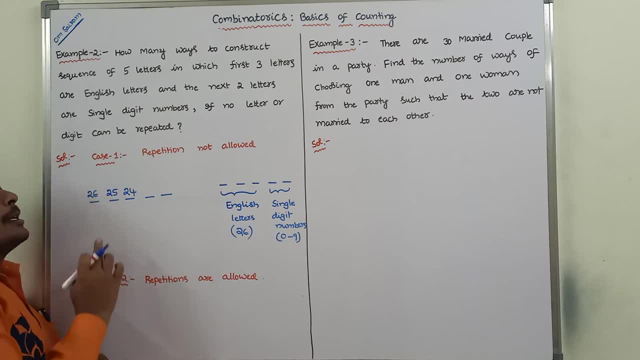 letter. one way is there for filling in that place, So that is 25 into 1, that is 25 ways. Okay. next, For filling the third vacant place, how many number of ways are there? Only 24,. 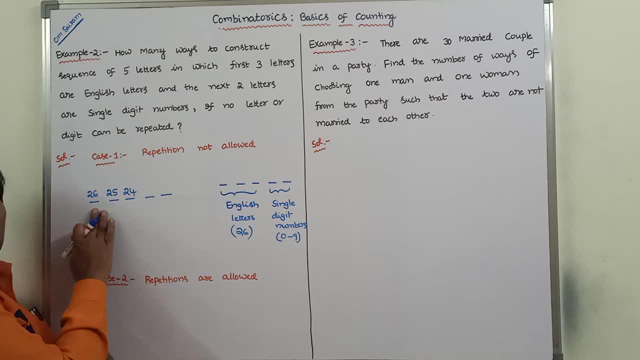 24 ways are there, because first two vacant places are filled with two letters. Okay, that two letters can be subtracted from 26 English letters. that is 24, because there is no repetition of any English letter is allowed, So that 24 letters are there For each and every letter. one way is there: 24. 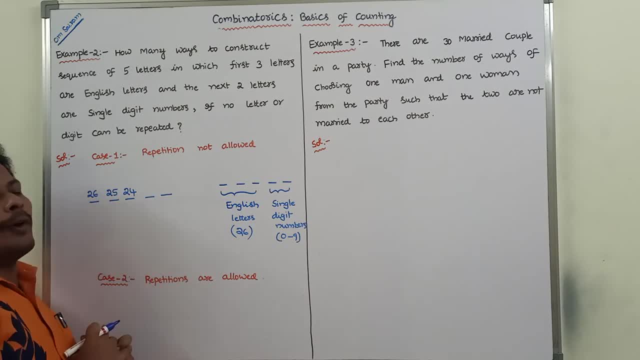 into 1, that is, 24 ways. are there Okay? so next one. Next two vacant places are filled with single digit numbers. Okay, single digit numbers are 0 to 9.. Total, so 10 numbers are there. Total 10 numbers are there, Okay? so for filling this vacant place. 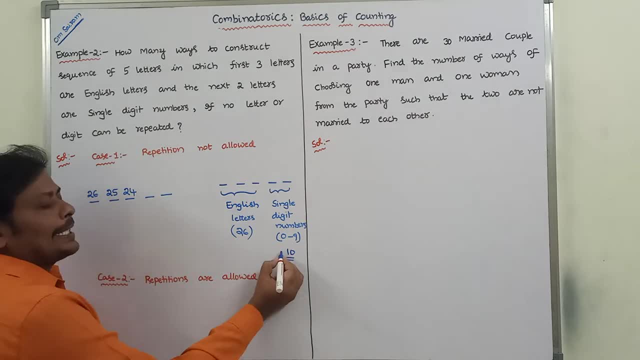 how many number of ways are there? Okay, so total 10 single digit numbers are there. Any single digit can be placed here. So that is 10 ways. are there? Next one? Next for filling out the last vacant place. how many number of ways are there? 10 ways. 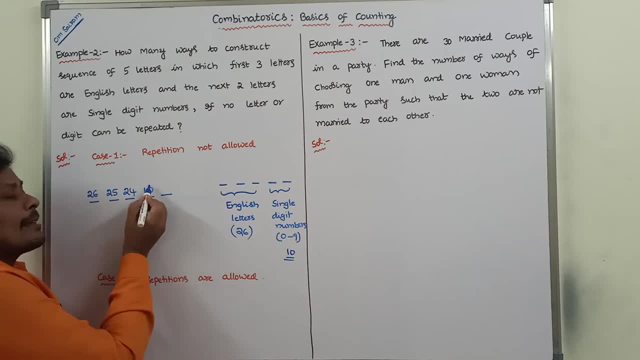 are there. Among the 10 ways, one digit is already filled in this place. Okay, that letter. that digit can be subtracted among the 10 numbers. 10 single digit numbers: Okay, only 9 numbers are there, So 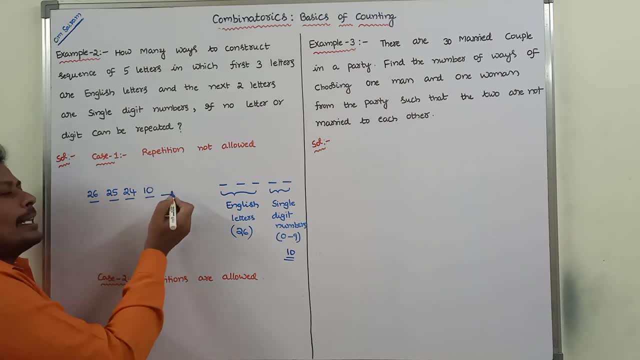 among the 9 numbers. we can place any number in this place. So 9 into 1, that is a 9. 9 ways are there? Okay, so total number: total possible number of ways is total possible number of ways is equal to 26 into 25, into 24, into 10, into 9.. 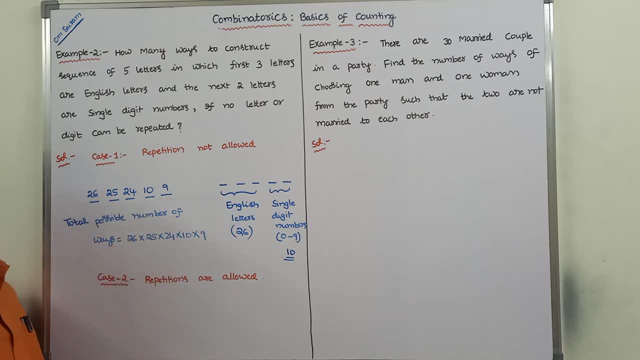 Okay, so this is the pearce column. Thank you very much, Thank you, Thank you, Thank you for watching, Thank you, Thank you, carefree. Such Aaah result okay. next, one second case: repetitions are allowed. so repetitions are allowed means: 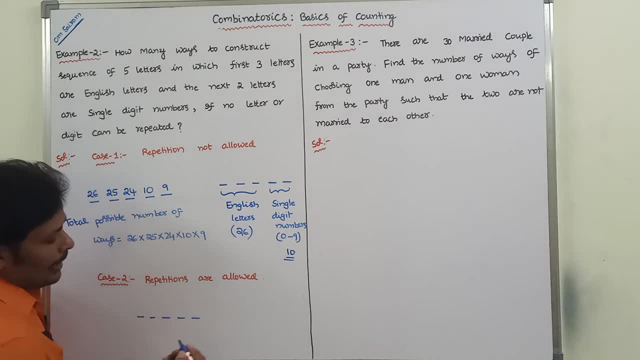 there are five vacant places, are there? okay? first, three vacant places are filled with the english letters. second, two vacant places are filled with the in single digit numbers. okay, for filling out this vacant place. so 26 english letters are there. so for filling out this vacant place. 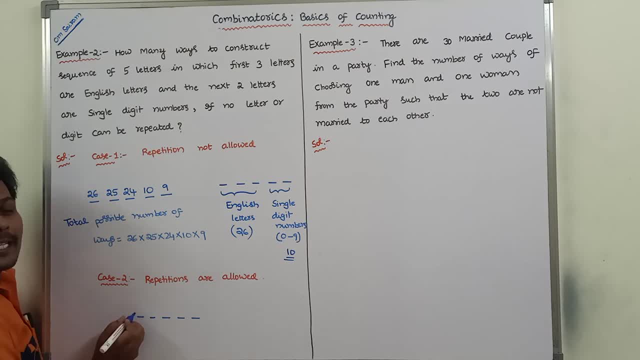 any letter we have to place. so how many number of ways are there? 26 ways are there, okay. next, for filling out the second empty space: okay. how many number of choices are there? so 26 choices are there. because there is a repetition of english letter, or? 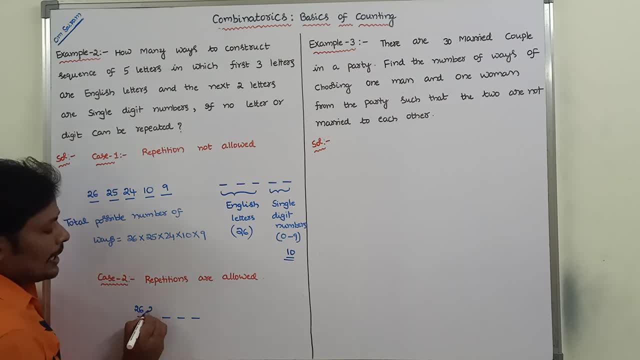 single digit number is there, so that so 26 choices are there for filling out the second vacant place. again 26 choices are there for filling out the third vacant place, because repetition is allowed. okay, here a is used, here also a is used, here also a is used, but here in that case there is. 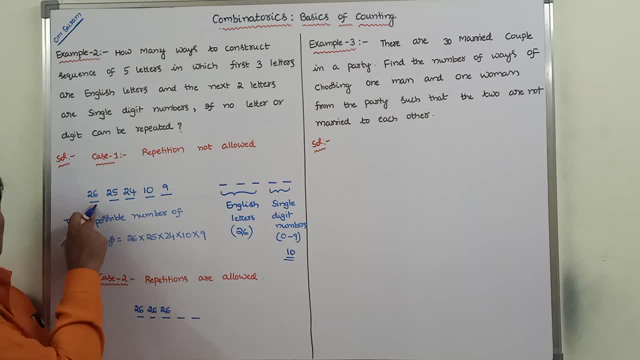 no repetition of any single letter here. a is used, here a is not used. here a is not used. okay. so in the same way, for filling out the fourth vacant place, so 10 single digit numbers are there. so for filling out this vacant place, so 10 choices are there, 10 ways are there? okay? 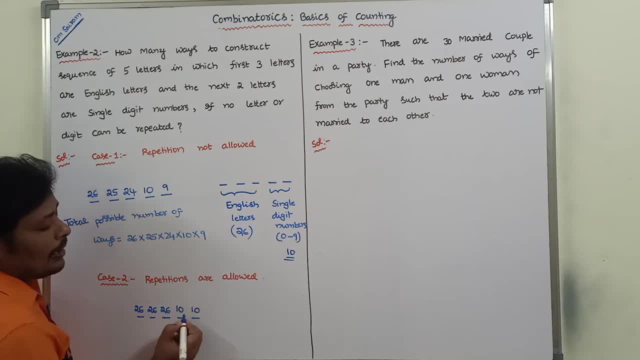 for filling out this vacant place. 10 choices are there because repetition is allowed, here and here, the same single digit number we are using because repetition is allowed. so therefore, of ways, total number of ways, total number of ways, possible ways, is equal to. so 26 into 26, into 26, into 10, into 10. okay, so this result will be: 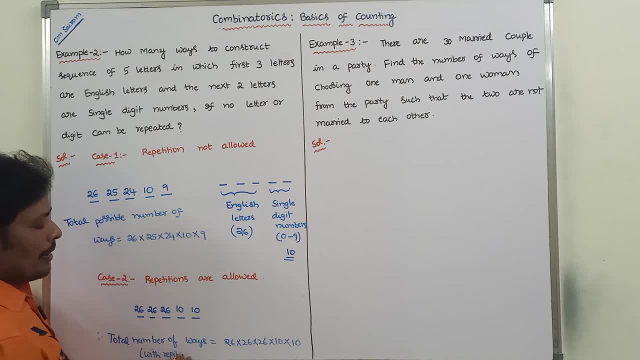 the repetition with repetition and repetition of R, Repetition of any single digit number. Okay, so here: repetition not allowed, Repetition Not allowed, Repetition not allowed. Okay, so next we go for next problem. The next problem is example 3. 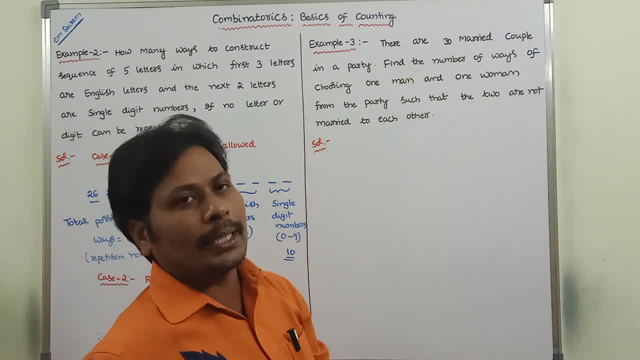 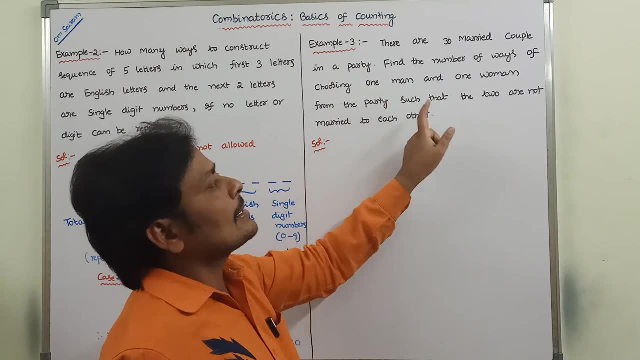 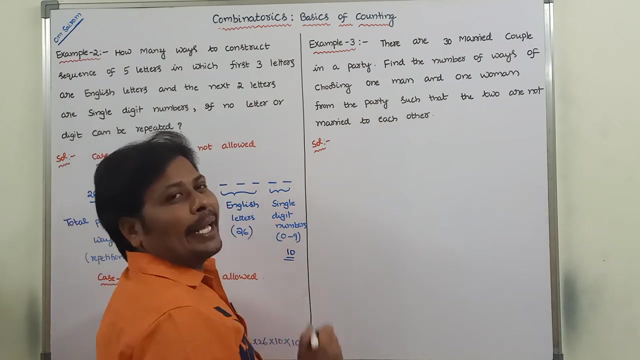 So there are 30 married couple in a party. Find the number of ways of choosing one man and one woman From the party such that the two are not married to each other. Okay, so here, 30 married couples are there. So among the 30 married couple, 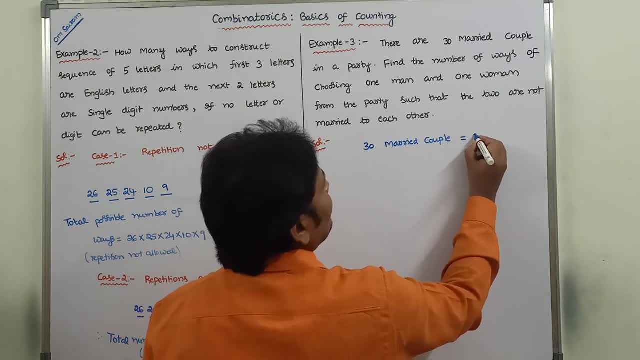 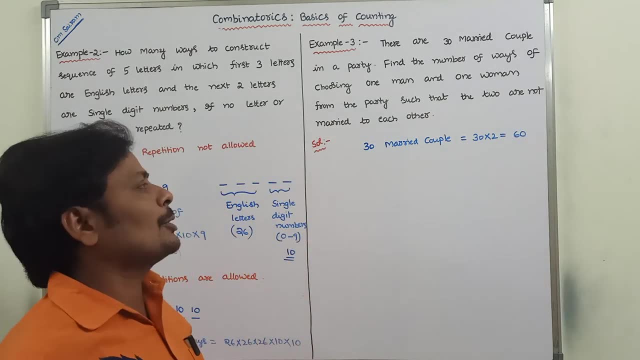 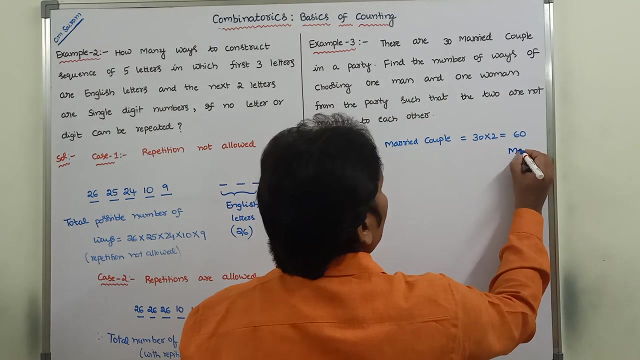 30 married couple. so total 30 into 2, because a couple is nothing but two persons. Okay, couple is nothing but two persons, one man and one woman. so Total is equal to: so 60 members. Total is equal to 60 members among the 60 members, So 30. 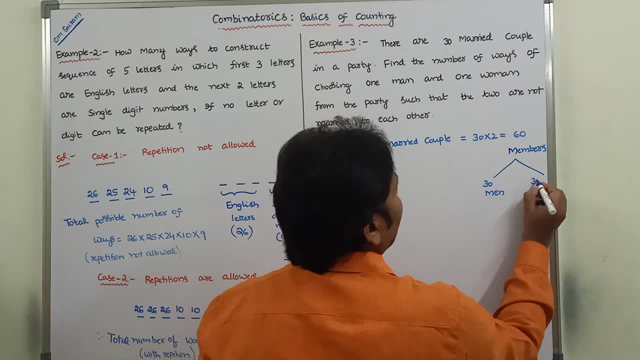 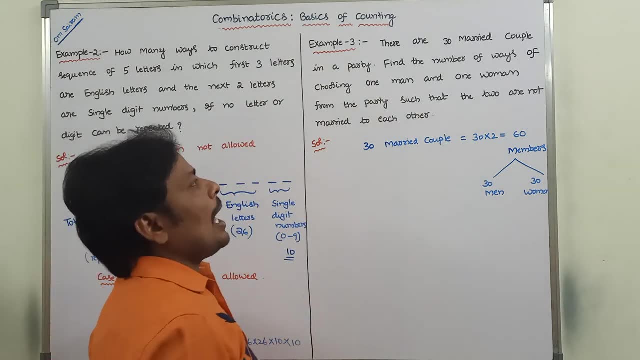 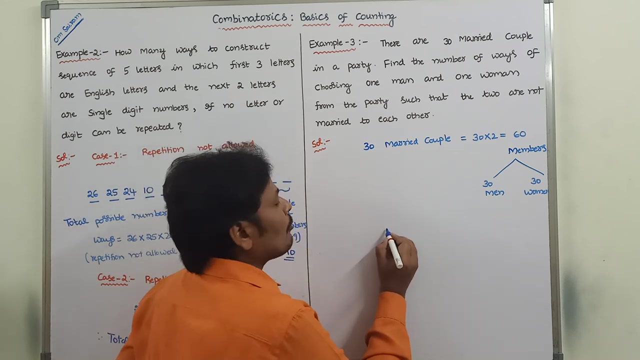 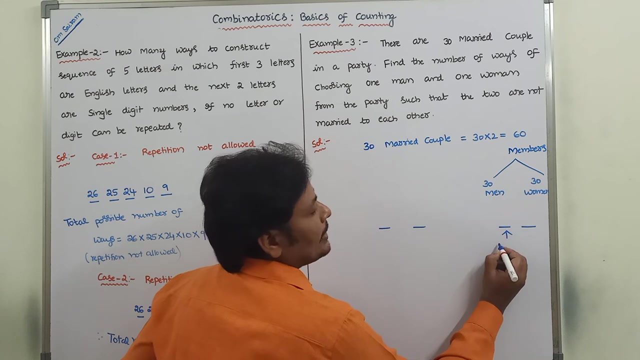 Man, 30 men and 30 women, 30 man and 30 women. Okay, So now I am taking, I am taking a couple. Okay, couple means two persons. couple means two persons: one man and women, one woman. so here, So the first vacant place allocated to man and the second vacant place can be allocated to woman. 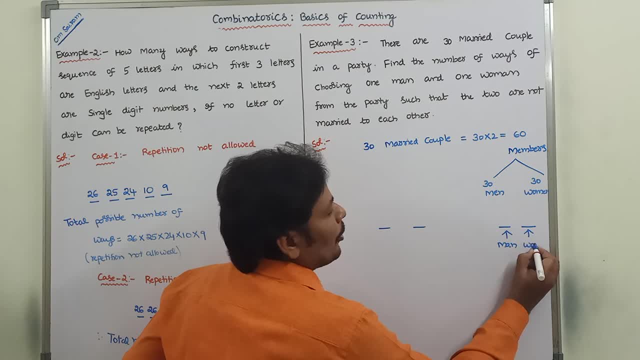 So the first vacant place allocated to man and the second vacant place can be allocated to woman. Okay, so how many number of man's are there? So 30 man, 30 men's are there and 30 women's are there. So total is 60 members. 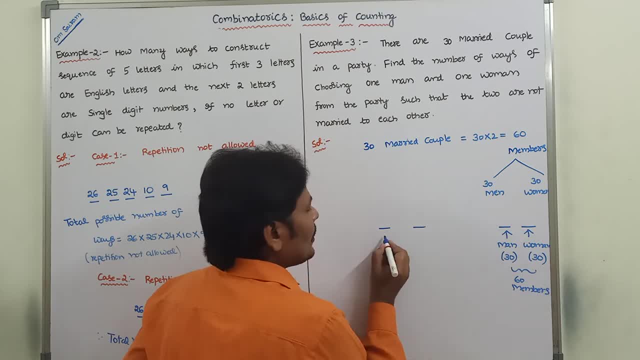 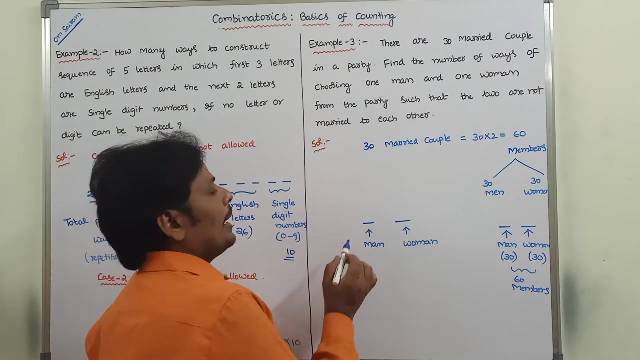 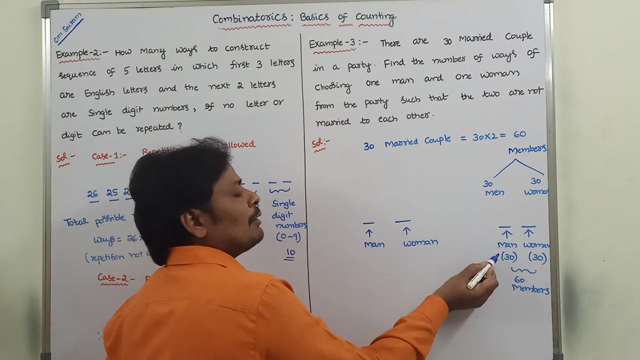 Total is 60 members. Total is 60 members. So this place can be allocated for man and this place can be allocated for woman. Okay, now, so far, placing a one man. Okay, one vacant place is there here. Total number of man: sir, This is 30. so for placing one man, one vacant place is there among the 30 men's? 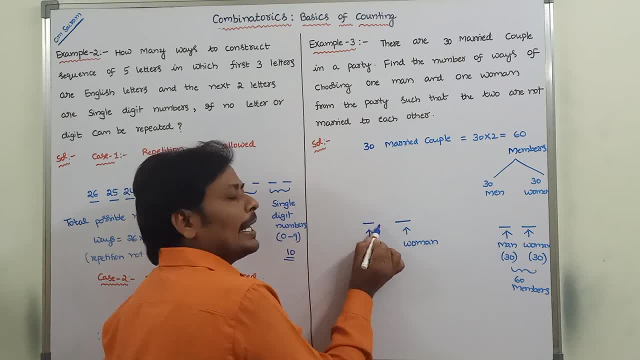 Okay, any man can allocated in this place. Okay, So that, how many number of face are there? So, for allocating 30 men in this place, there are. how many number of face are there? 30 base are there. Okay, Next one. 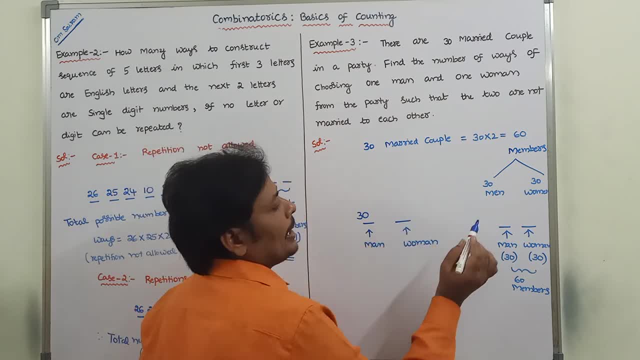 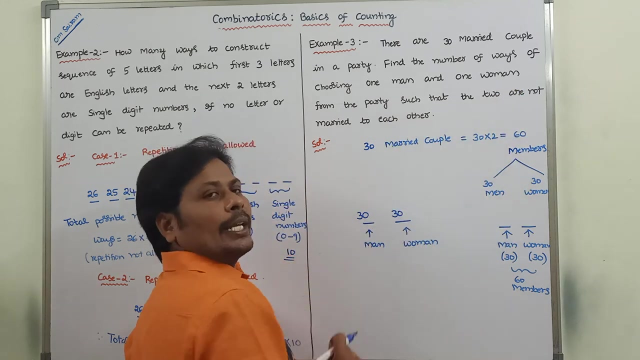 So here we are placing women's. Okay, Here, 30 women's are there. Okay, 30 women's can be placed in this one, Okay, Okay. But here the condition is the two members are not married to each other. Okay, Here, one man is there, That man has the wife in that place. Or one woman is there That woman?